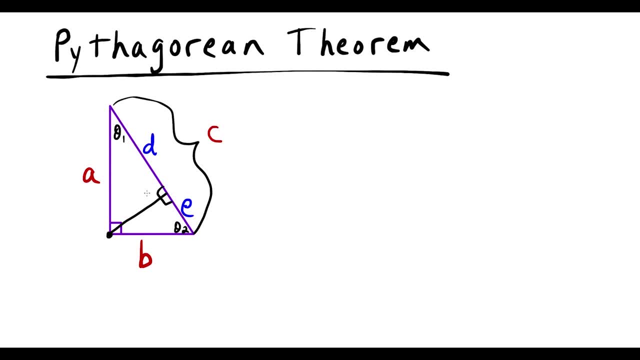 theta one plus theta two is going to equal 180 degrees. So if we look at this medium size triangle right now, we have 90 theta one. This would have to be theta two. And then in the small right triangle we have 90 theta two. This would have to be theta one, And note here that theta one. 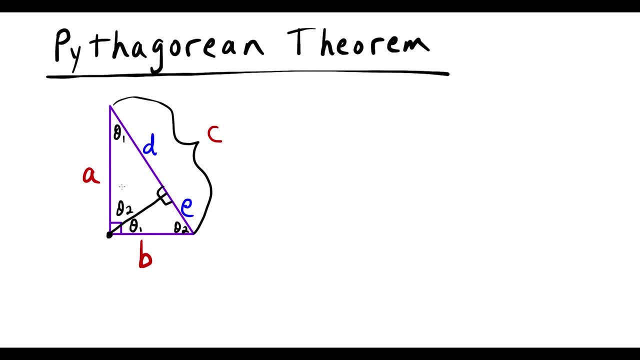 plus theta two equals 90. So this is all checking out So far. we have three similar triangles. Now the first proportion I want to set up here is: I'm going to look at the first, I'm going to look at the big right triangle And I'm going to set up the ratio A over theta two And I'm going to set up 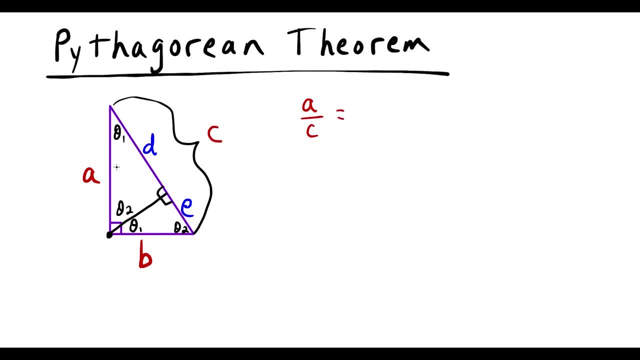 A over C. So we're going to have A over C equals, and I want to compare it to the medium triangle. But be mindful, in the big triangle A was a leg and C is the hypotenuse, But in this medium size triangle D is the leg, So I'm going to write D over here, over the hypotenuse of the medium size. 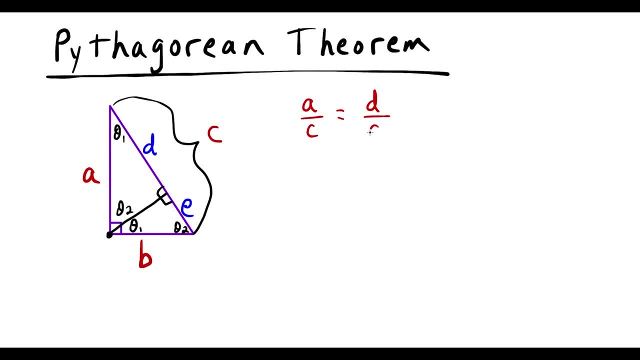 triangle is A because it's across from the right angle, like this. Now, the next thing I'm going to set up is the next triangle here, the small one. What I'm going to do is I'm going to compare it to the big triangle And I'm going to set up the ratio A over C And I'm going to set up the. 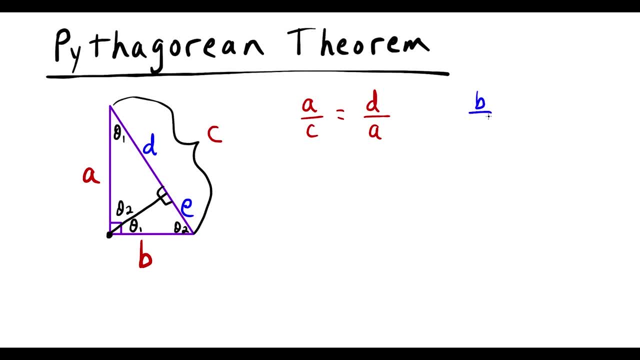 ratio B over C. So that's the other leg compared to the hypotenuse of the big triangle. But now in the small triangle, the other leg here is E over the hypotenuse of the little triangle is B, because it's across from this right angle like this. So this ratio we'll definitely check out. So now 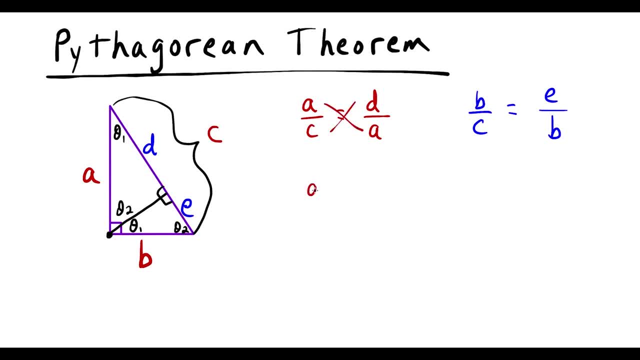 what we're going to do is we're actually going to cross multiply like this, And this is going to give us A squared equals and we're going to have C times D. But then when we repeat this process in the second proportion, we have B times B is B squared. 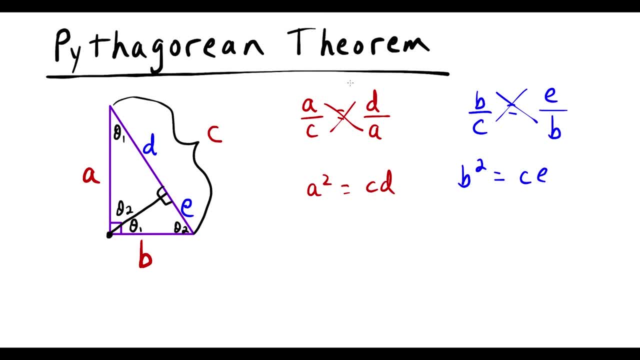 And that's going to be equal to C times E. So now what I want to do is I'm going to actually add these equations together, So I'm going to have A squared plus B squared. I'm going to add the left side, So I have A squared plus B squared And that's going to be equal to the sum of the. 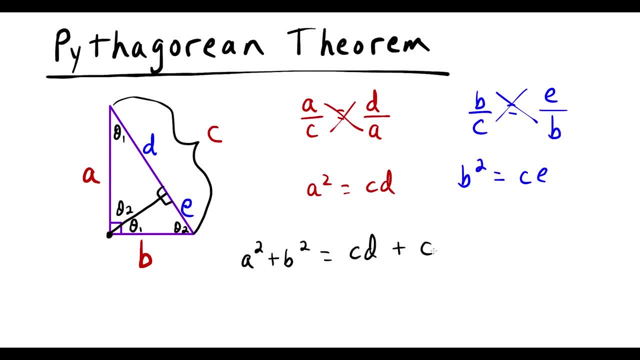 right side. So I'd have C times D plus C times E. But notice, we could factor here To add this, we could factor out a C And this is going to leave us with D plus E. And now you may not seem, it may not seem like we accomplished much here, but we have A squared plus.